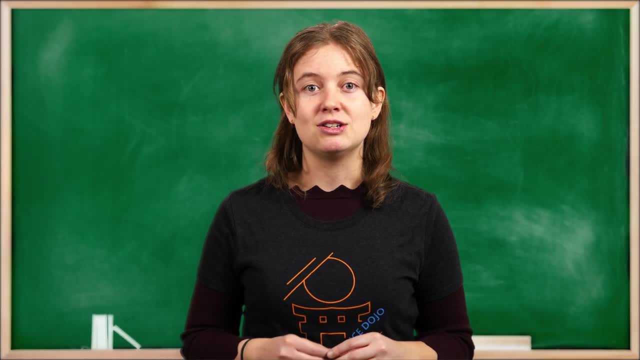 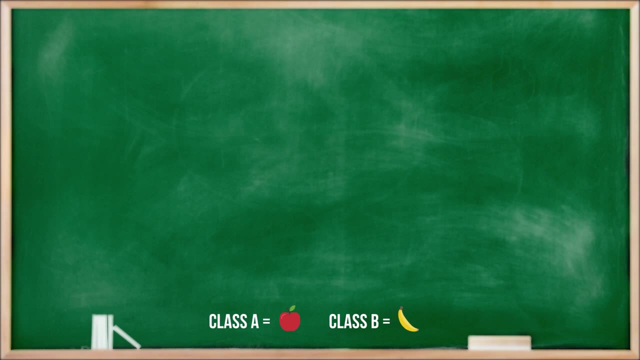 Recall and F1 measure different things, so let's break it down into each of their parts and the role each play in measuring a model's accuracy. Let's say your classification model predicts apples and bananas. If your model avoids a lot of mistakes in predicting bananas and apples, then your model has a high precision. Likewise, 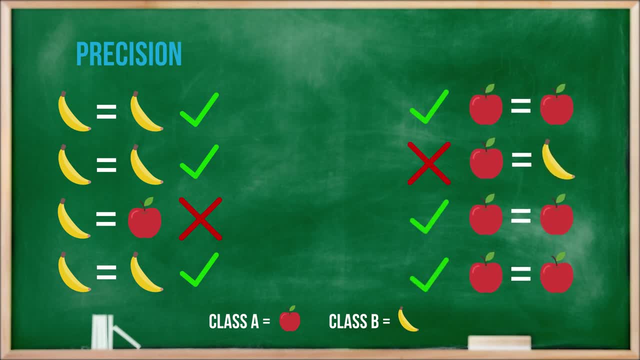 if your model avoids a lot of mistakes in predicting apples and bananas, then your model has a high recall. You want your model to aim high for both precision and recall, where your model avoids as many mistakes as possible, doing a good job at correctly predicting both. 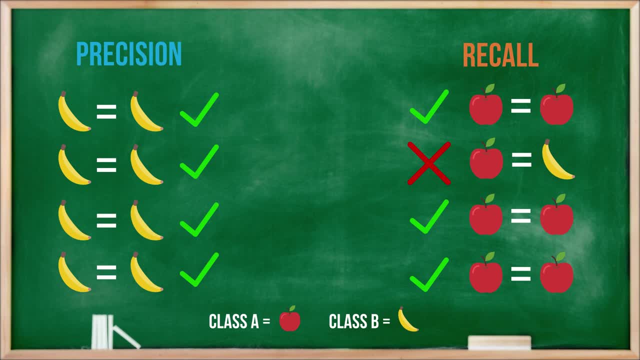 apples and bananas. But what if your model aces the fidelity to predict one class? Wouldn't it be misleading to look at precision or recall in isolation? This is where F1 comes in. It takes into account both precision and recall. A balance of the 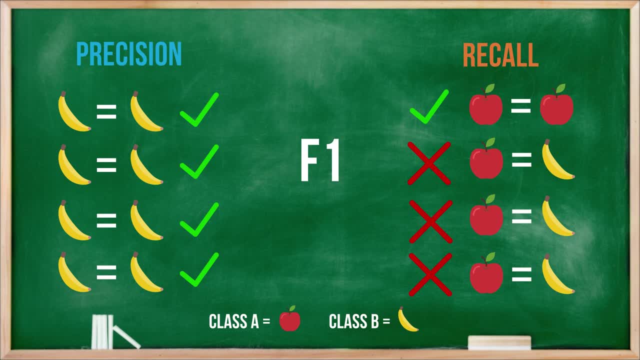 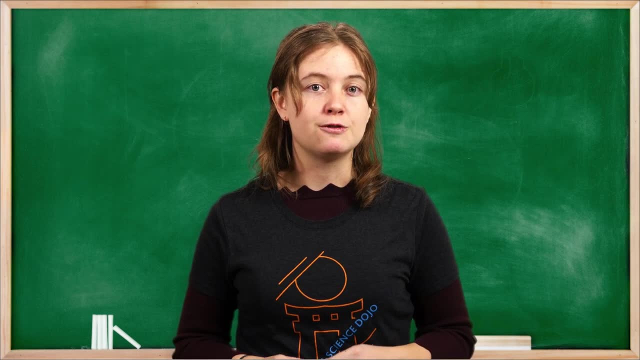 two is what F1 scores on. If your model does a good job at accurately predicting both apples and bananas, then it will have a high F1 score. There are some cases where you might focus on precision more so than recall, and vice versa. For example, Class A might be an aggressive 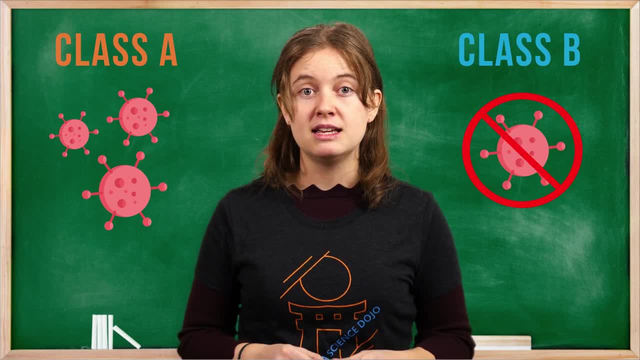 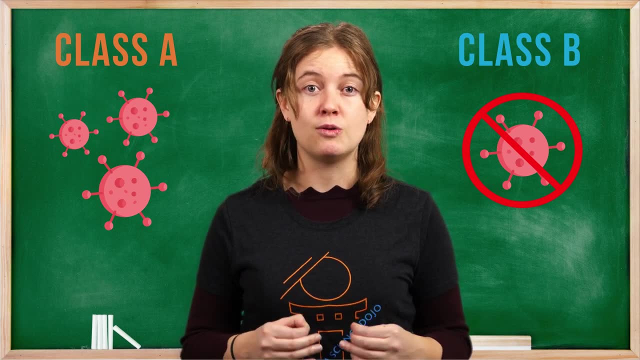 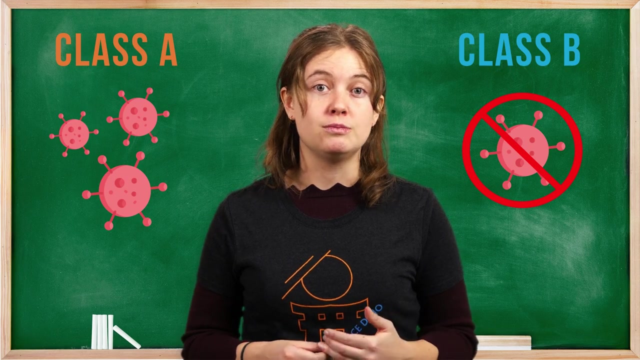 type of cancer and class B might be no cancer. The stakes of misleading cancer as no cancer or overlooking the cancer can be extremely high. Therefore, you want your model to avoid mistaking cancer for no cancer or mistaking A for B. This means you want to focus on recall. 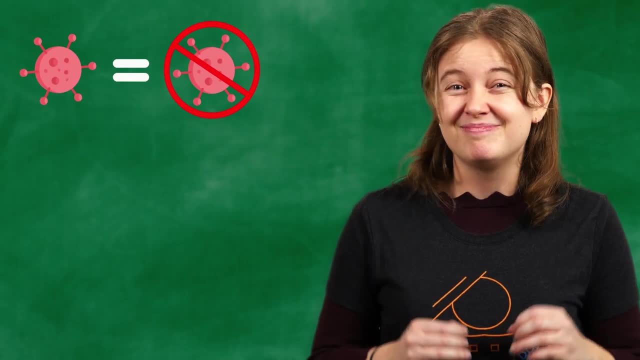 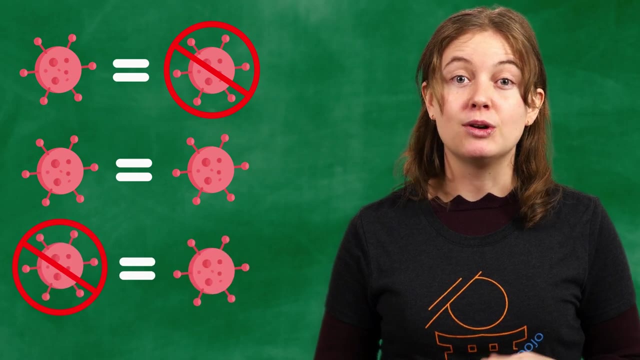 You don't want your model to say, whoops, I missed the cancer, sorry. You want your model to say I got the cancer. maybe I was overly cautious and had mistaken a few. no cancer patients for cancer patients. but isn't it better to have a false alarm of? 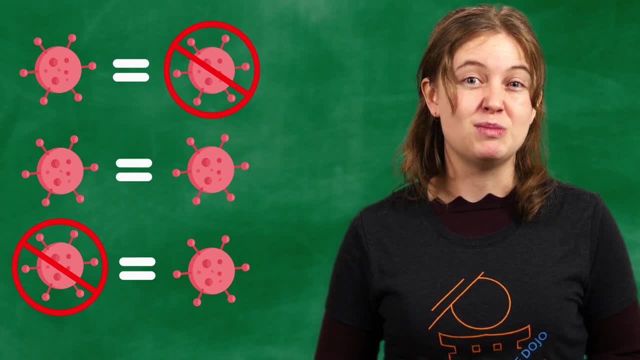 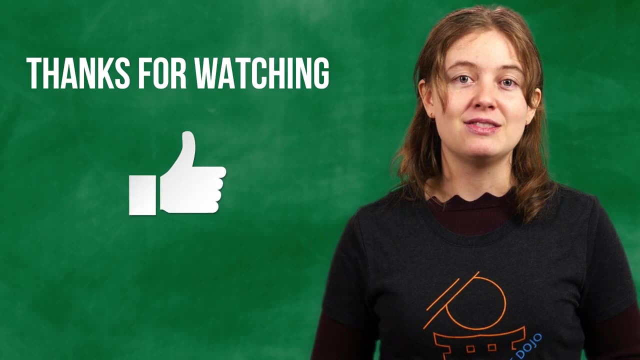 you don't have cancer after all, rather than sorry, you actually do, but we missed it. And that sums up precision, recall and F1.. Thanks for watching. Give us a like if you found this useful, or you can check out our other videos at Data Science Dojo Tutorials. wwwdata-sciencecom.